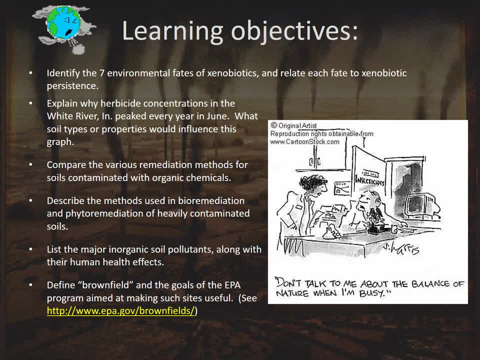 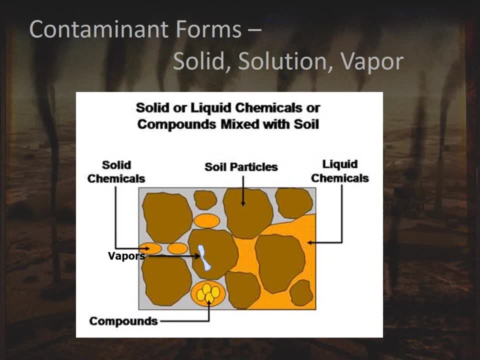 human health effects associated with them, And we're going to learn what a brownfield is. So contaminant forms in soils come as either solids, a solution, or effluents, vapor, and they can be associated through soil pores or the services of soils. the 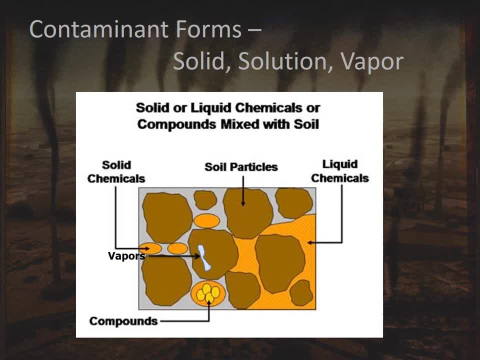 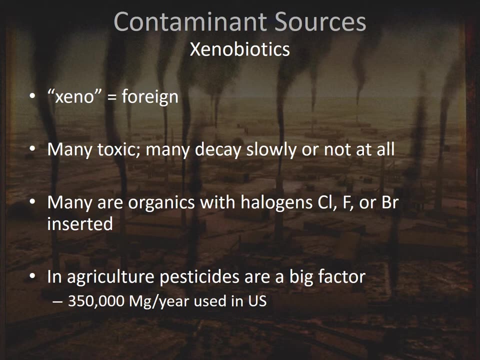 same way, any of the nutrients we discussed can be associated with them. it can be adhered to the surface via adsorption or can be absorbed into the actual structure, loosely associated, so contaminant sources. we're going to talk about something called xenobiotics. xeno basically means foreign, so a xenobiotic. 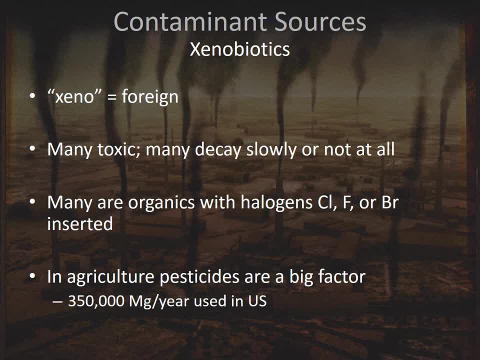 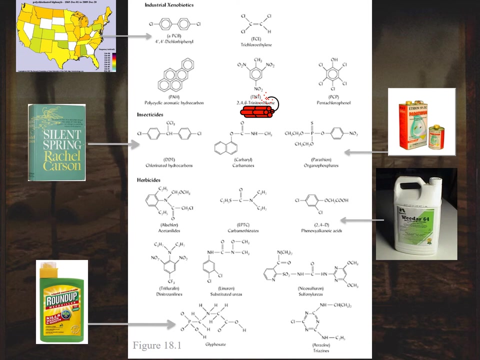 is basically anything foreign that's introduced to the soil. that's bad, all right. so most of these are toxic and they decay very slowly or not at all. some of them are organics with halogens inserted of them. some of them are agriculture pesticides. these are a very big factor. here's some examples: you 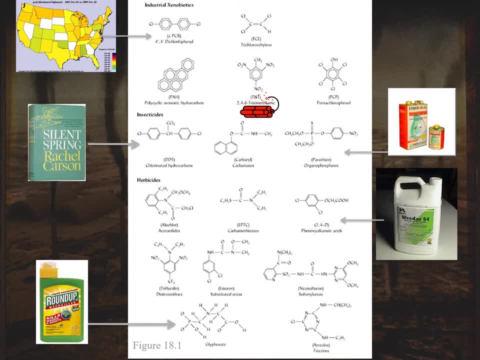 do not need to know these chemical structures. this is just kind of a cool little graphic I put together to. to give some examples: PCBs are an example. TNT, you know, like the song, TNT, your dynomite- well, that is a xenobiotic as well. parathon is is a great example. 2 to 4 D is something that we add to. 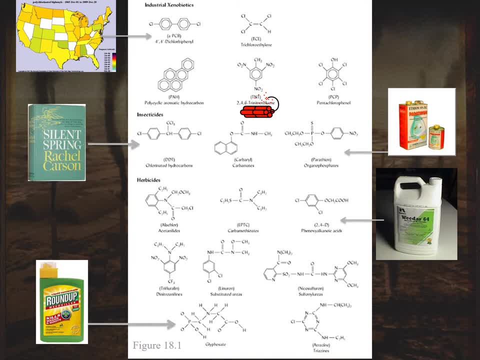 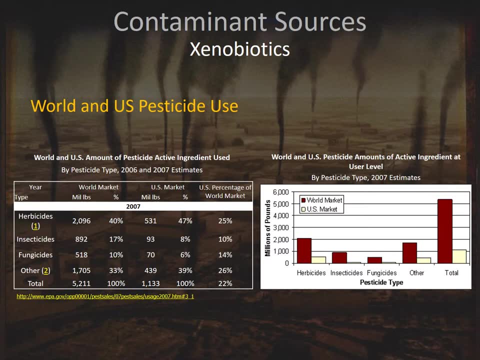 example 2 to 4 D is something that we add to. example 2 to 4 D is something that we add to to kill weeds um, you know there's roundup. glyphosate is is an example. atrazine is another weed killer. um world and us pesticide use has has basically been increasing for a long time. 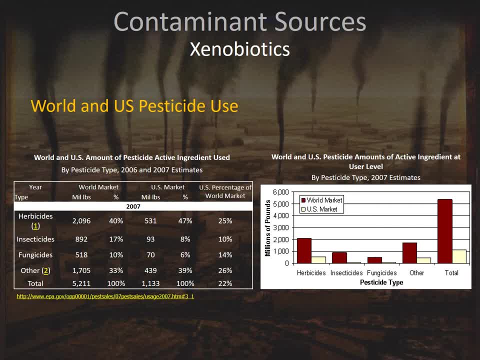 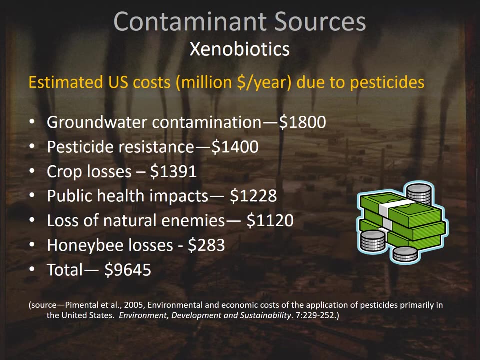 this is a grave concern. we've got herbicides, insecticides, fungicides- all these things are definitely a concern, but more so on the world market than on the us market. the world market's using a lot more than we are, not to say that we aren't causing either. 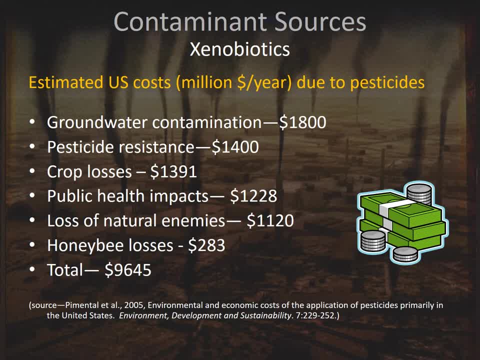 we're going to talk about. the estimated united states costs a million dollars per year due to pesticides. in the united states alone, groundwater contamination per year costs us 1800 million dollars per year. pesticides resist- pesticide resistance: 1400 million dollars a year. crop losses: almost 1400 million dollars a year. public health impacts: 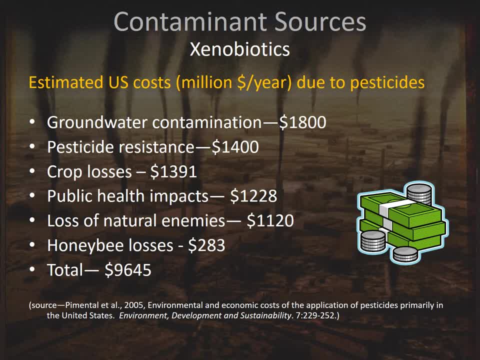 you a little over 1200 million dollars a year loss of natural enemies- which is a part of the importance of the ecosystem, like praying mantises and and brachinoid wasps, which help to um decrease the amount of predatory insects. so the loss of these natural enemies is costing us about 11. 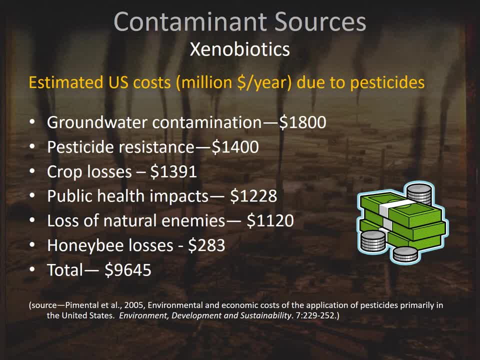 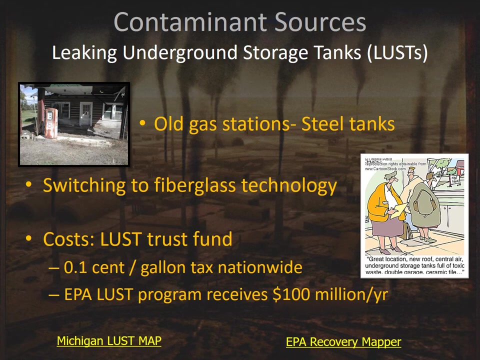 1100 million dollars a year. honeybee losses about 283 million dollars a year. uh, in total, we're we're losing about 9600 million dollars a year due to pesticide use. so this is the grave concern we need to pay attention to. another thing that i want to teach you guys about is um leaking underground storage tank. 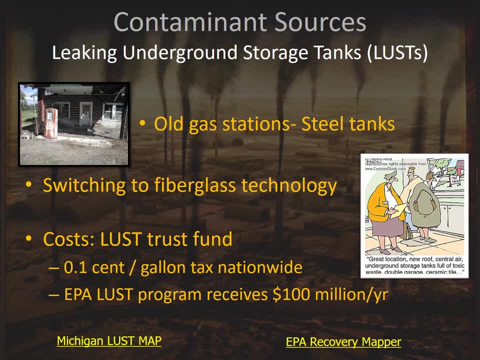 all right. so these are from old gas stations, where we used to store on the petroleum or the gas in steel tanks underground. well, the thing about steel tanks is they rust and link, all right, and so we need to pay attention to this, And so we've switched to fiberglass technology now to stop this from happening. 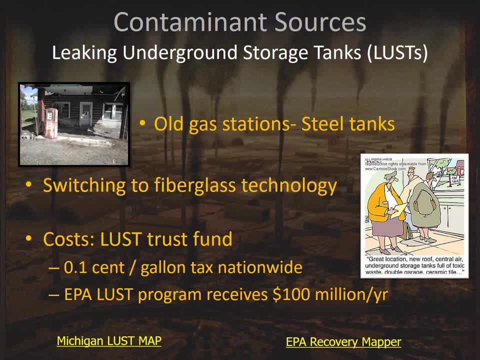 However, we still have a bunch of these old leaking steel tanks underground everywhere, And so we created something called the Lust Trust Fund, where 0.1 cent per gallon of tax nationwide goes into this program to help address these issues. So let's look at Michigan, which has a lust map. 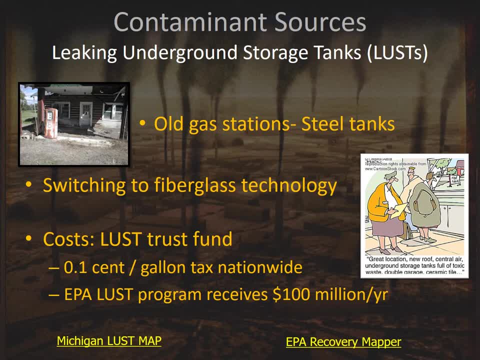 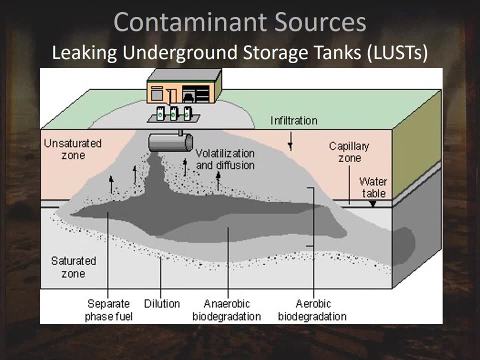 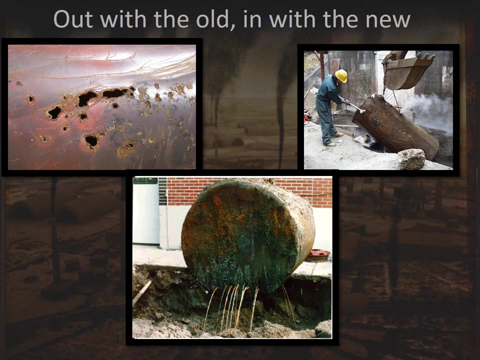 There's goats screaming in the background- Totally normal. So what happens is that leaking tank leaks gas into the underground environment and this contaminates the water table. Here's what a leaking underground storage tank looks like when it's being pulled out of the ground, just to give you a nice little visual of how bad this is. 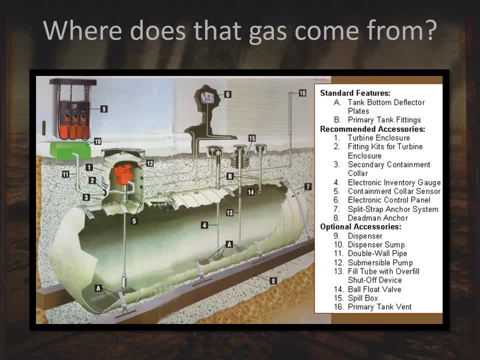 So here's kind of the makeup of the tank. You don't need to know this, It's just kind of information, Because I didn't know this until I looked at one of these diagrams, kind of understanding how the gas comes out of the tank underground and into the pump and then therefore into your vehicle. 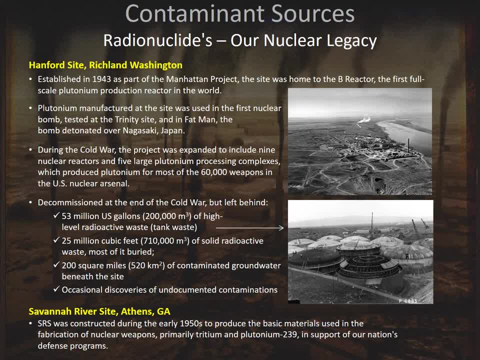 There's another issue we need to talk about that can contaminate soil, and those are radionucleotides. So we have this really cool nuclear legacy, And by really cool I mean not cool at all. The Hanford site in Richland, Washington, was established in 1943 as a part of the Manhattan Project. 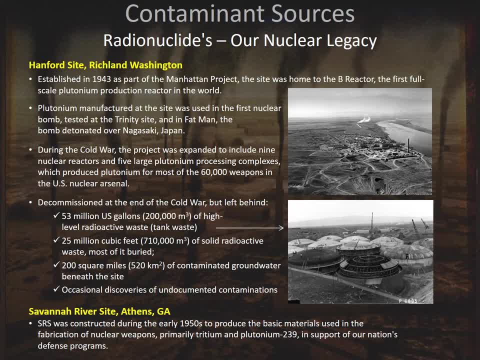 So this site was home to the B Reactor, which is basically the full scale Plutonium production reactor in the world. So plutonium was manufactured at the site or was in the first nuclear bomb which was tested at the Trinity site and in Fat Man, which was what was detonated over Nagasaki, Japan, during the Cold War. 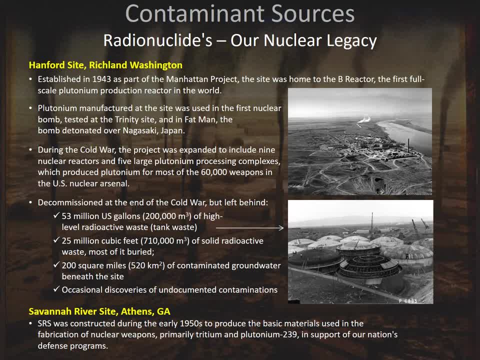 The project was expanded to include nine nuclear reactors and five large plutonium processing complexes, and this produced plutonium for most of the 60,000 weapons in the US nuclear arsenal. We decommissioned this site at the end of the Cold War. 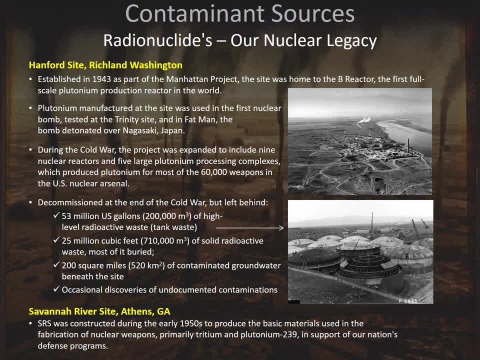 But even though we decommissioned it, it left behind some presents. It left us 53 million United States gallons of high-level radioactive waste. It left us 25 million cubic feet of solid radioactive waste, most of it which we buried, 200 square miles of contaminated groundwater beneath the site and occasional discoveries of undocumented contaminations. 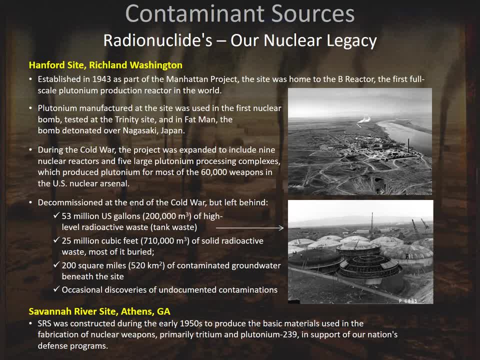 Because the thing about top secret sites like this is: nobody tells anybody. It's the truth. There's also a Savannah River site in Athens, Georgia, and I actually was supposed to work here, but I took this job instead. SRS, which is what I'll refer to, the Savannah River site, as was constructed during the early 1950s to produce the basic materials used in the fabrication of nuclear weapons. 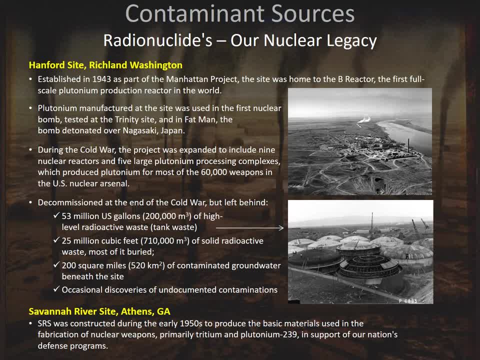 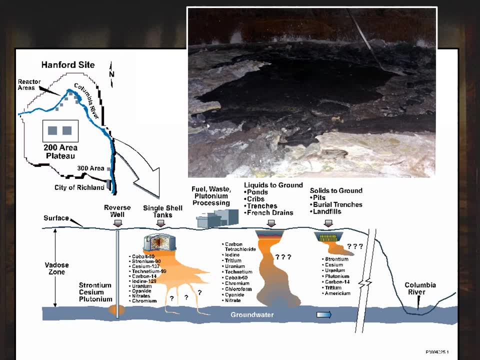 Primarily they produced tritium and plutonium-239 in support of our nation's defense programs. So, talking about that, The Hanford site, The reactor, is right next to the river. They're always next to a source of water because you have to use water to cool the reactor. 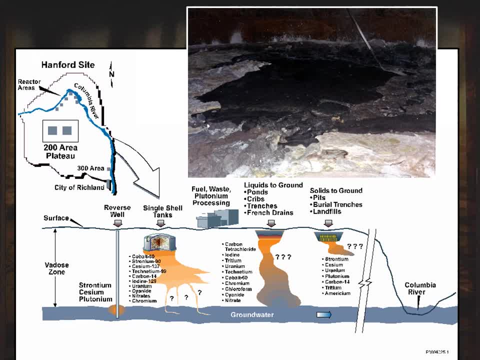 And when you don't, it melts down. That's basically what happened during the tsunami in Japan a few years back. was that, even though they're right next to the ocean, because the tsunami destroyed everything, they were unable to pump water into the reactors to cool them down? 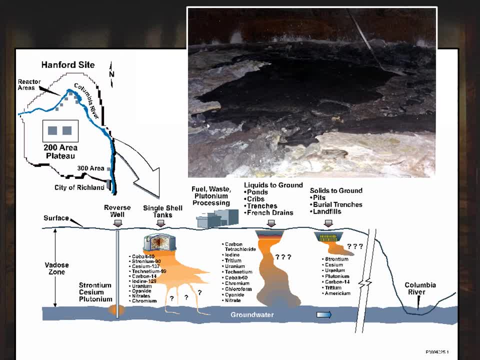 And then it melted And then we have worldwide radioactive contamination. So here at the Hanford site we have the Columbia River right next door to the reactors to help cool them down, But the surface we have single shell tanks that are ultimately leaking cobalt, strontium, cesium. 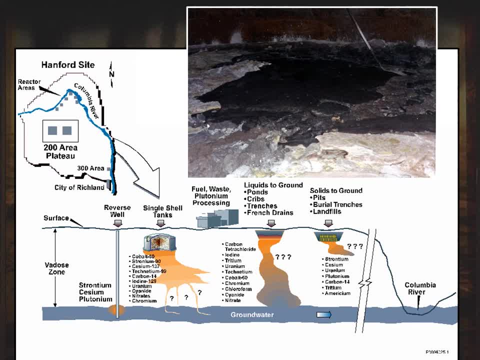 technetium, carbon-14,, iodine-129,, uranium, cyanide, nitrates, chromium and other special things that we don't even know about. We have fuel, waste, plutonium processing, which ultimately leads to liquids to the ground from ponds, cribs, trenches, French drains. 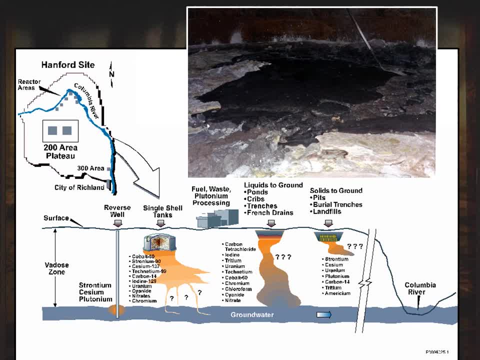 where we get carbon, tetrachloride, iodine, tritium, uranium, technetium, cobalt-60,, chromium, chloroform, cyanide and nitrate leaking into groundwater. We also have solids to the ground from pits, burial trenches and landfills. 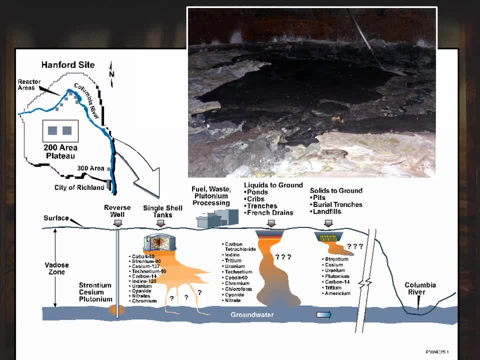 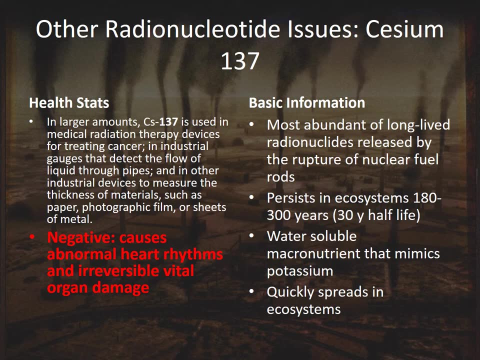 They're resulting in leaking strontium, cesium, uranium, plutonium, carbon-14, tritium and americium leaking into groundwater. None of this is good folks, So some other radionucleotide issues include cesium-137.. 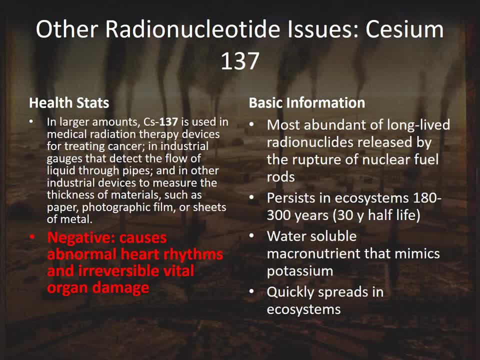 So in large amounts. cesium-137 is used in medical radiation therapy devices for treating cancer, In industrial gauges it detects the flow of liquid through pipes and in other industrial devices. it basically measures the thickness of materials such as paper, photographic film, sheets of metal. 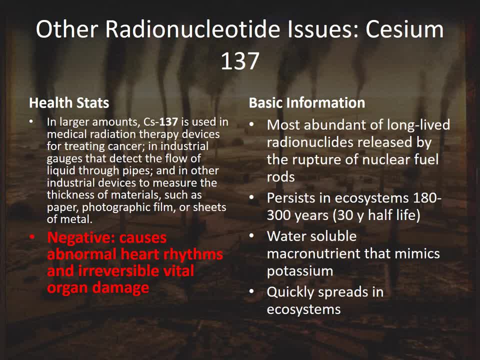 The negative here is that it causes abnormal heart rhythms which can cause cervical-vital organ damage. Basically, we have the most abundant of long-lived radionucleotides here. It's released by the rupture of nuclear fuel rods and it persists in ecosystems. wait for it: 180 to 300 years, because that's a 30-year half-life. 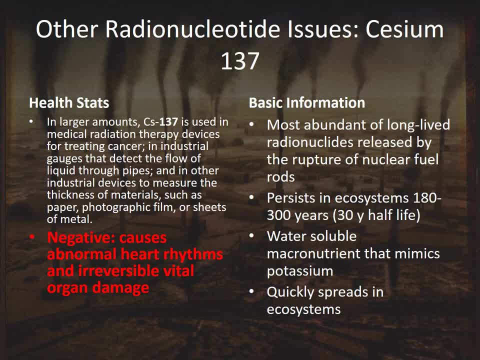 It's water-soluble. It's a water-soluble macronutrient that mimics potassium. So wherever potassium goes, cesium-137 goes, because it pretends to be. it imposter And it quickly spreads in ecosystems because of this. 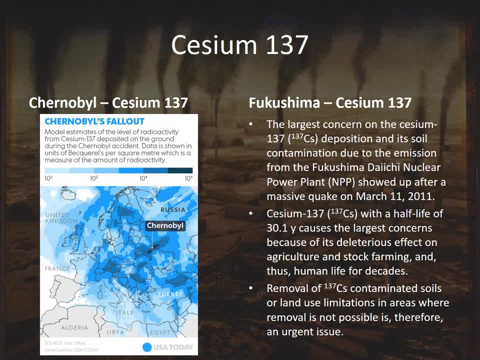 So one example of this was in Chernobyl, as well as in Fukushima. So let's talk about Fukushima, since this is the most recent catastrophe involving this. The largest concern on the cesium-137 deposition and its soil contamination is due to the emission from the Fukushima nuclear power plant. 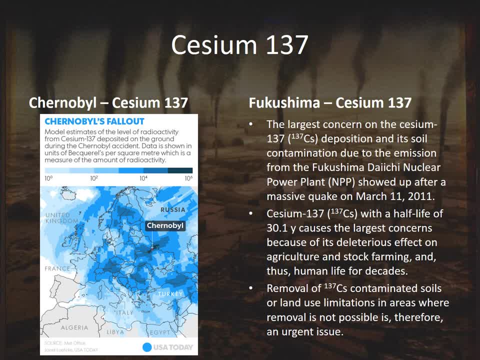 We basically saw this showing up after a massive quake on March 11th in 2011.. Cesium-137 has a half-life of 30.1 years, so it causes the largest concerns because of its deleterious effect on agriculture and stock farming, and thus human life for decades. 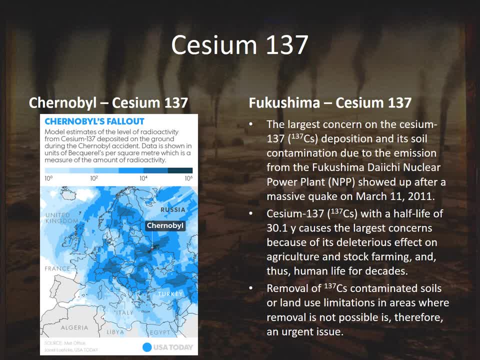 So it just it lasts forever. So the removal of cesium-137 from contaminated soils or land use limitations in areas where removal is not possible is an urgent issue. We need to get rid of it. How Where do we go? 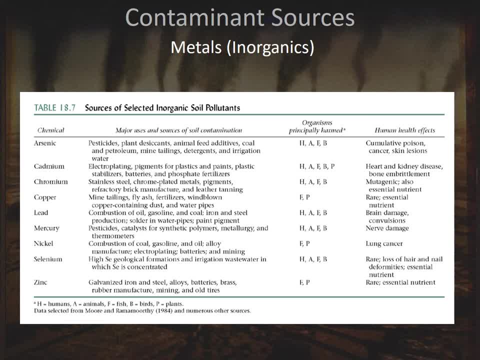 All right. so there's some other inorganic pollutants like metals that we need to talk about. So arsenic is what I studied in grad school. We see it in pesticides, plant desiccants, animal feed additives, coal, petroleum mine tailings, detergents, irrigation water. 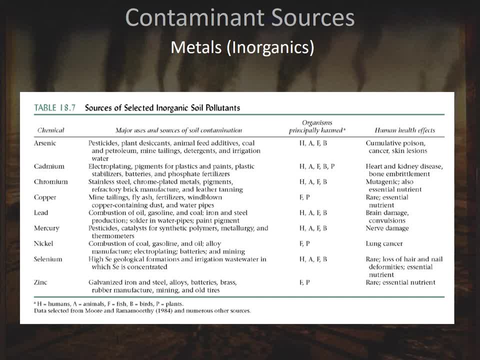 It's a cumulative poison that causes cancer and skin lesions. Cadmium- we see this in electroplating pigments for plastics and paints, plastic stabilizers, batteries, phosphate fertilizers- causes heart and kidney disease and bone infertilement. chromium, stainless steel, chrome plated metals. 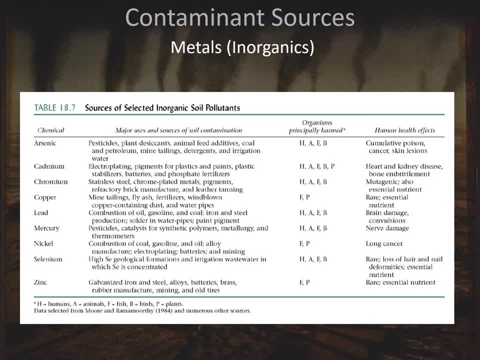 pigments, refractory brick manufacturing and leather tanning. We see this is immunogenic. It's also an essential nutrient. so that's fun Copper. we see this in mine tailings: fly ash fertilizers, windblown copper containing dust and water pipes. 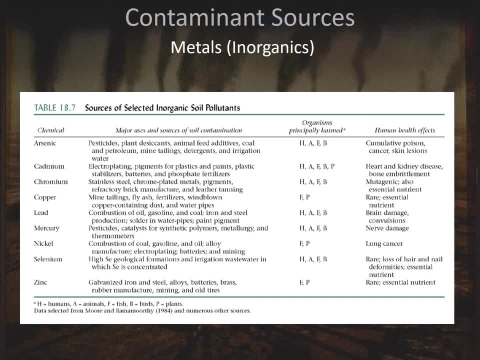 This is a rare essential nutrient, Lead. lead is something that we're studying in Muncie on a grand scale, which is of grave concern. It's from combustion of oil, gasoline and coal. It's from iron and steel production. We see it in the soldering- soldering in water pipes. 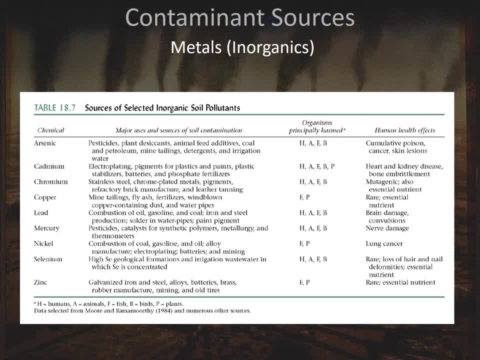 although it's not allowed to be used in water pipes anymore, We do still see it as in soldering at certain water pipe jointing. So it's not as much of an issue anymore, But in older homes it still exists in the pipes. 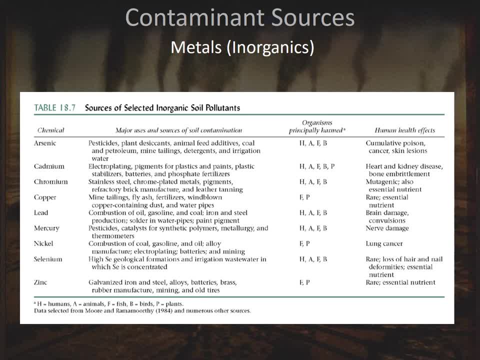 And that is a problem. It's a paint pigment. We don't use lead based paint anymore, but we still have a lot of lead based paint in in homes. It's not usually removed, It's usually just painted over. So you know, when you rent a home and they give you that lead paint disclosure. 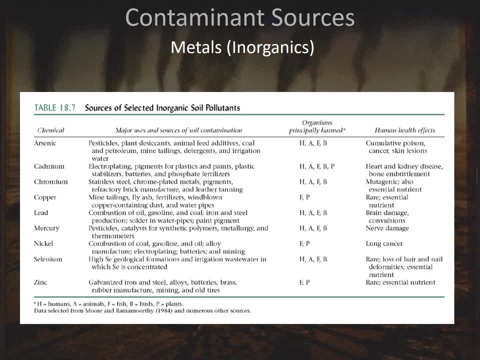 the problem with lead is it causes brain damage. So essentially, what lead does is it's a neurotoxin and it can build up in your bones because it mimics the. I think it mimics calcium, if I remember correctly. So it builds up in your bones. 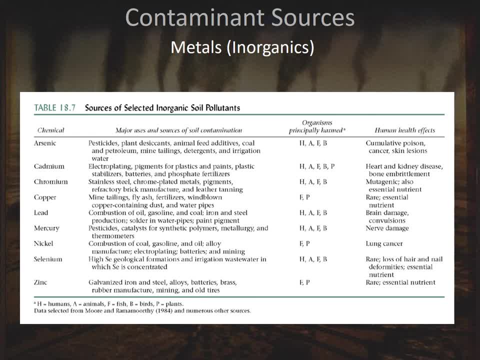 But while it's in your, while it's in your bloodstream before it builds up in your bones, it basically makes you stupid, All right. So it binds all of your neurotransmitters and and it basically makes it so you can't think normally, And so we're seeing a huge issue with this in kindergarten issues. 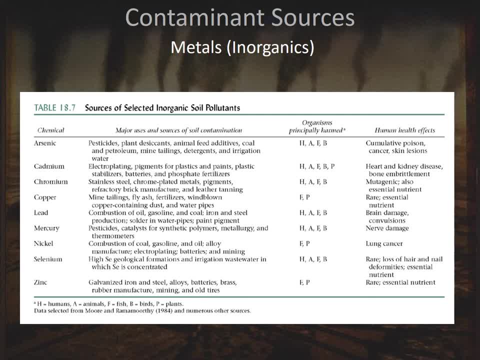 You know. so people who are growing up in households that are high in lead content are having a harder time learning basic things, and this may be resulting in concentrated populations basically having a negative impact on their ability to learn and succeed in life. And, of course, we tend to see high lead levels in areas where we have 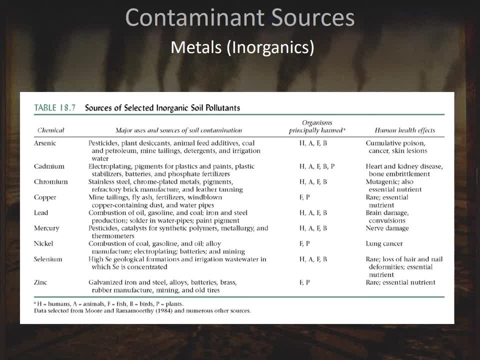 older homes and therefore lower income status, And so the problem perpetuates. mercury: We see this: It's a catalyst for synthetic polymers, metallurgy and thermometers, and it causes nerve damage. Nickel, And we see this in the combustion of coal, gasoline and oil. 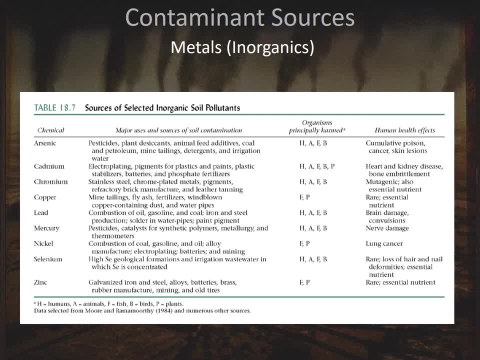 Alloy manufacturing, electroplating, batteries and mining causes lung cancer. Selenium: We see high selenium geological formations and irrigation wastewater in which selenium is concentrated. It has rare human health effects, but it can cause loss of hair and nail deformities, And it's also an essential nutrient. 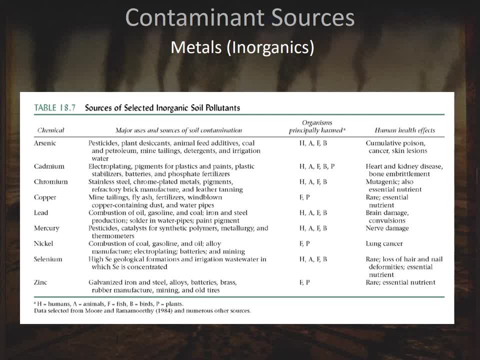 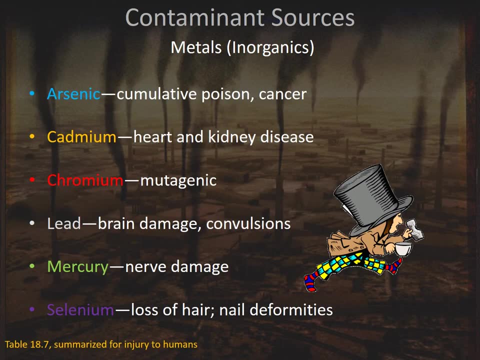 But in in too high a quantity it causes issues. Zinc is used in galvanized iron and steel, alloys, batteries, brass, rubber manufacturing, mining and old tires. It has rare human health effects because it's an essential nutrient, but it can still cause. 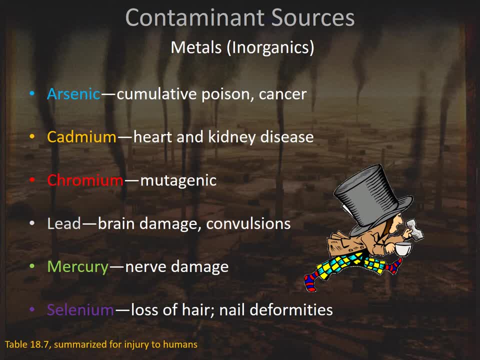 So some of those metal inorganic contaminants: arsenic causes accumulative poisoning and cancer. cadmium causes heart and kidney disease. Chromium is immunogenic. Head causes brain damage and convulsions. Mercury causes nerve damage. Selenium causes loss of hair and nail deformity. 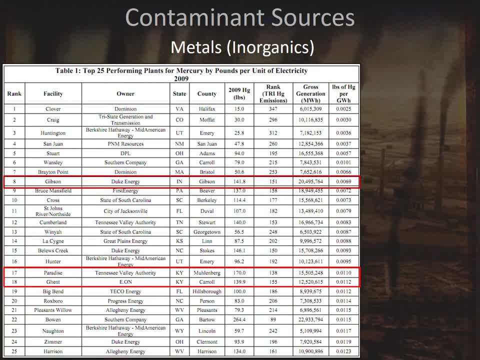 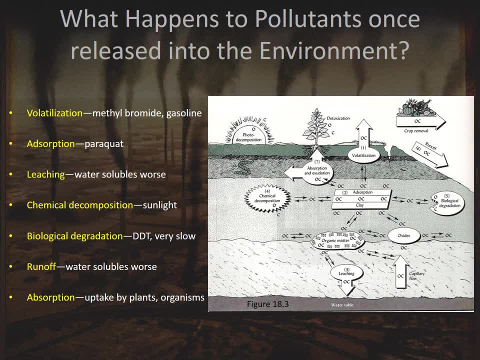 So we want to make sure these things aren't. I'm going to skip this one. skipping, skipping, skips, All right. So what happens to our pollutants once they're released into the environment? Well, methyl bromide and gasoline, for example, usually volatilize to the atmosphere. 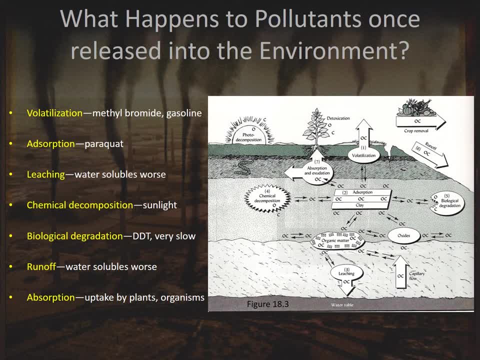 They may absorb to the surface of the soil, like paraquat, which is something that can absorb to the surface of soil. We might see them leach into groundwater. Things that are water soluble are really bad at this. They do it a lot. 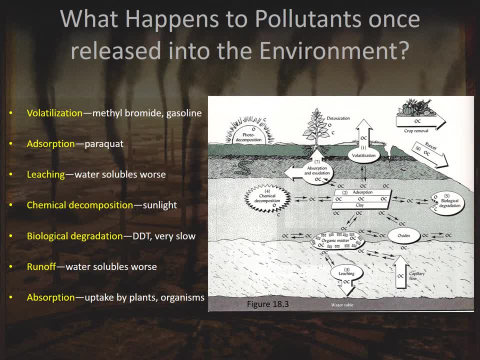 Chemical decomposition might happen. So sunlight in this instance is a good thing, because it decomposes it usually into a less toxic form. It might biologically degrade. So DDT, for example, can biologically degrade, but it takes a really long time. 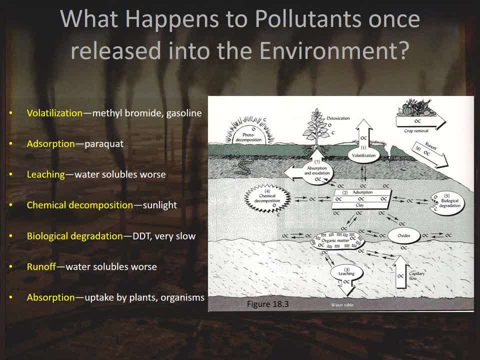 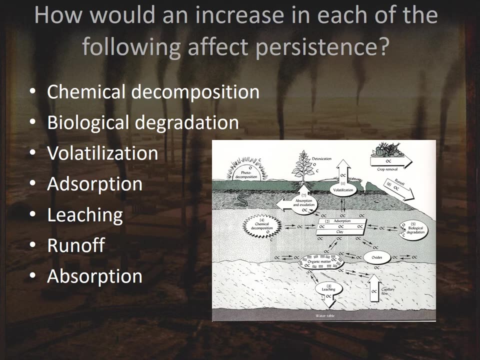 It might run off. It might degrade into surface waters, which is a problem, And water solubles are definitely of greater concern for this. It might absorb, be uptaken by plants and organisms, which can be a problem, for you know the things that eat them and move up through the population. 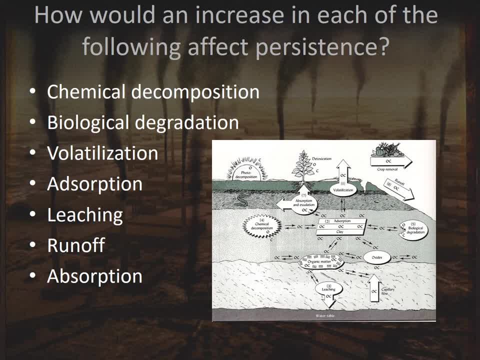 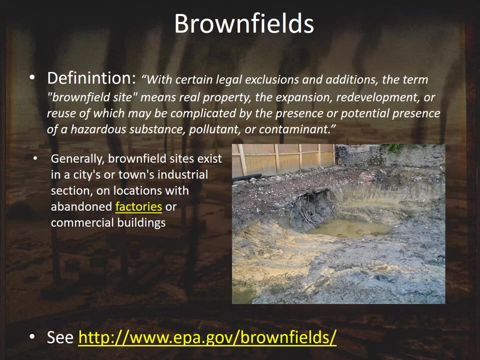 Bioaccumulation. So how would an increase in each of the following affect persistence? You know, chemical decomposition, biological degradation, volatilization, off absorption, all of these things can go on to cause issues in other parts of the ecosystem. 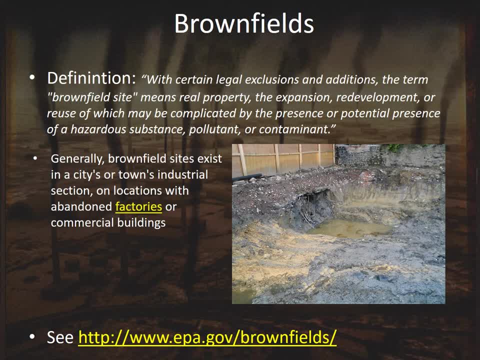 We're going to talk about brownfields. We have a lot of brownfields in Muncie. Brownfields by definition, with certain legal exclusions and additions. the term brownfield site basically means a real property of the expansion, redevelopment or reuse of which may be complicated by the presence or potential. 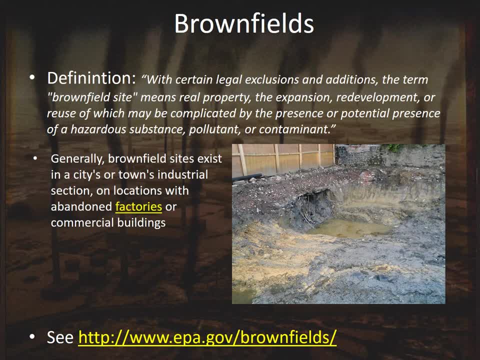 presence of a hazardous substance, pollutant or contaminant. Generally, brownfield sites exist in a city's or town's industrial section near, like an abandoned factory or commercial buildings, And so Dr Pichetel teaches a lot of classes where they go out and they fix brownfields. 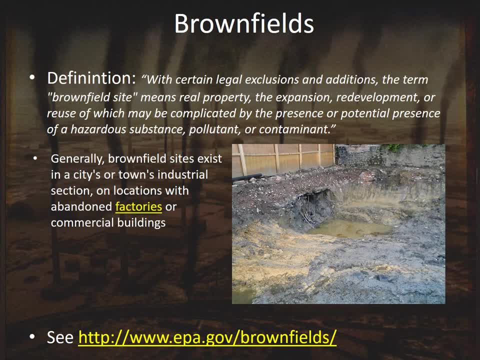 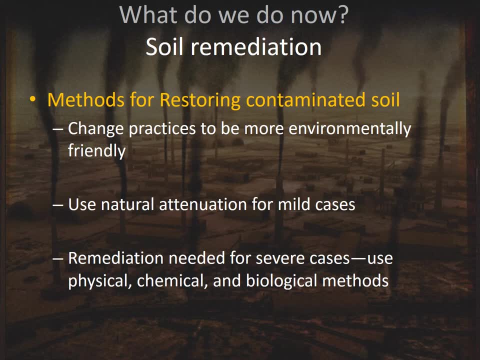 They turn them into a remediated park, for example. Soil remediation is basically a method for restoring contaminated soil, And so we're basically changing the practices there to be more environmental friendly. Sometimes we use natural attenuation for mild cases, which basically means we let nature take its course. 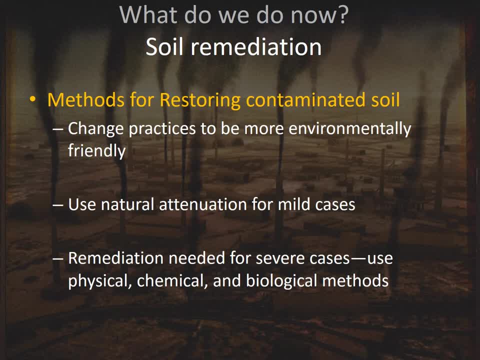 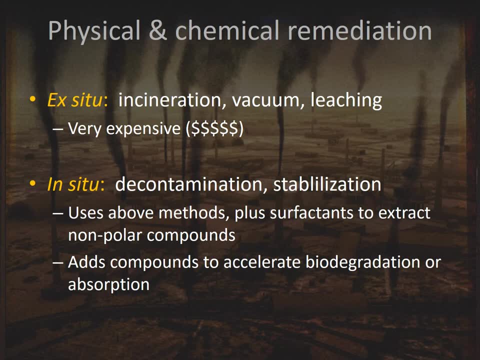 However, remediation may be needed for severe cases where we need to use physical, chemical and biological methods to clean up the soil. So ex-situ remediation is where we incinerate, vacuum or leach away whatever the problem is, and this can be very expensive. 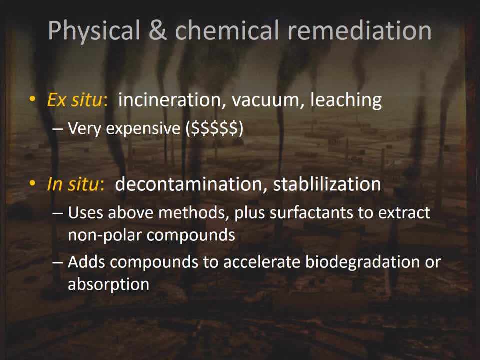 In-situ, however, is where we decontaminate, stabilize. We can use some of the above methods, above methods plus surfactants, to extract nonpolar compounds and then treat them, or we can add compounds to accelerate biodegradation or absorption, basically cause the the toxic chemicals. 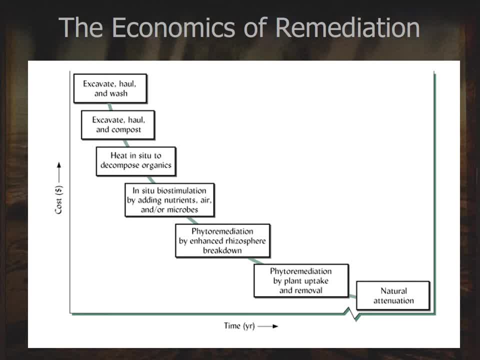 to turn into something non-toxic. There's a cost associated to this and there's a time factor. So excavating, hauling and washing soil is going to be very expensive, but it doesn't take much time. Same thing with excavate haul and compost. 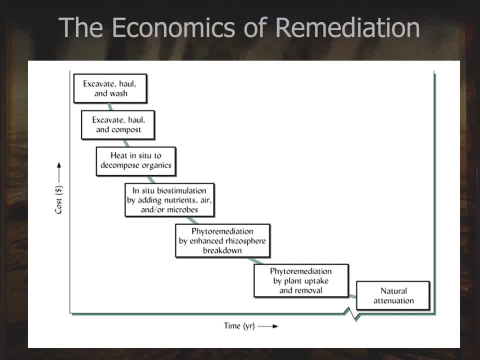 We can heat things in place to decompose organics into less toxic forms, or we can cause biostimulation by adding a nutrient, some air or some microbes to help degrade faster. Phyto-remediation may enhance rhizosphere breakdown. 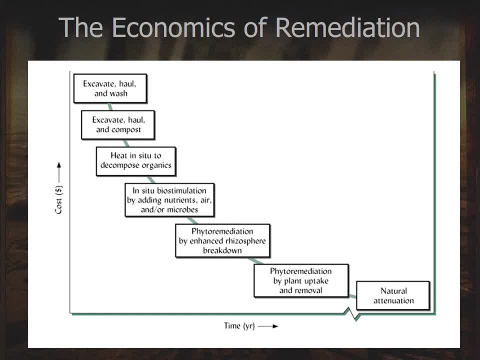 Phyto-remediation by plant uptake and removal. However, we have to be attentive to where we put those plants that we remove, because they are now stock full of whatever compound we took out of the soil And you only phyto-remediate the depth of the roots. 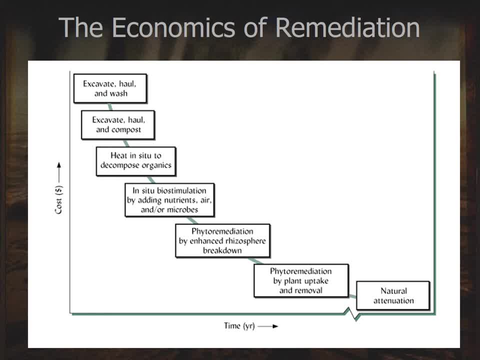 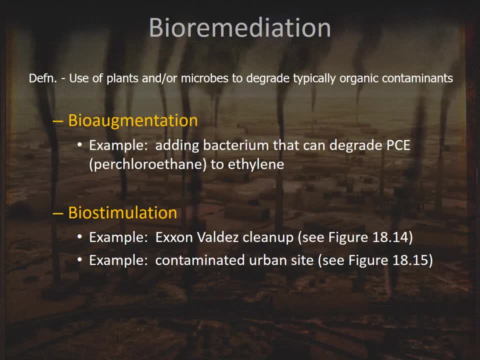 So if your contamination goes deeper than the roots, you also have to address that, in addition to phyto-remediation or natural attenuation, which takes a long time but is very cheap, All right. so bioremediation, by definition, is the use of plants and or microbes. 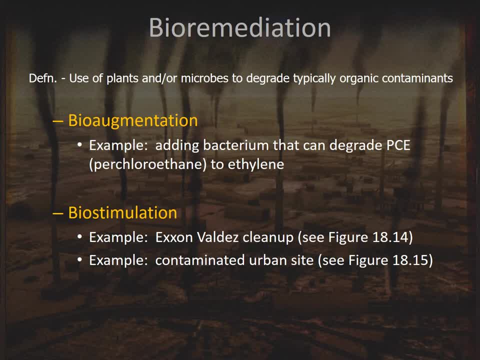 to degrade typically organic contaminants. Bio-augmentation, for example, could be adding bacterium that can degrade PCE perchloroethane to ethylene, which is considered to be less toxic. Biostimulation is where we add something to stimulate cleanup. 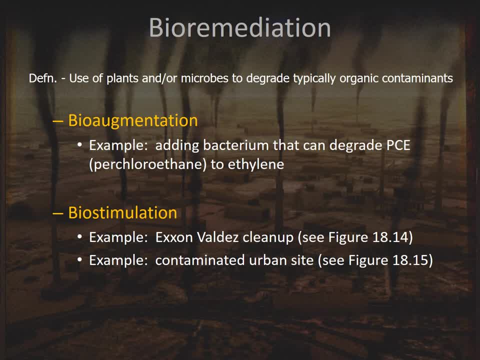 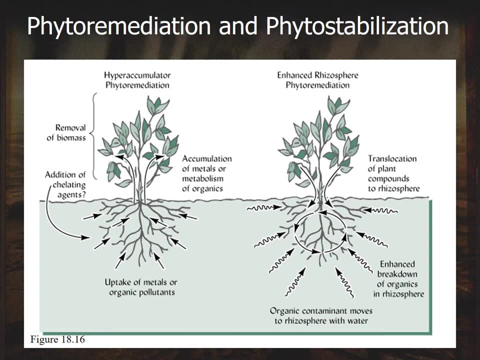 So Exxon Valdez used this, The contaminated urban sites also. Phyto-remediation is basically where you plant a plant that hyperaccumulates whatever thing is there. it basically sucks whatever contaminant into the plant tissues and then you remove the plant. 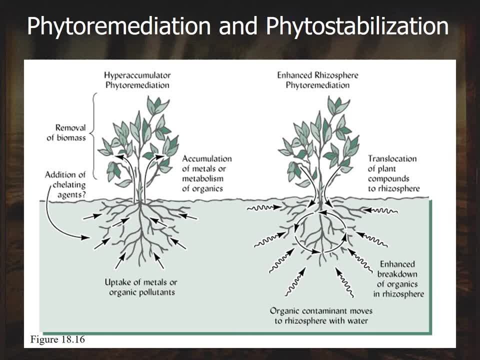 and you take it somewhere where it can be incinerated or safely decomposed. But again, it only addresses the depth of the roots. So remember, if you're using phyto-remediation, you need to test how deep your contamination goes, because it may need to be paired with something else. 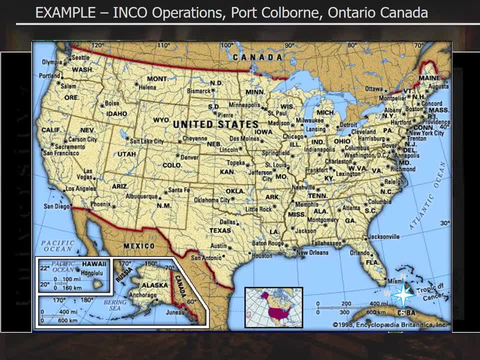 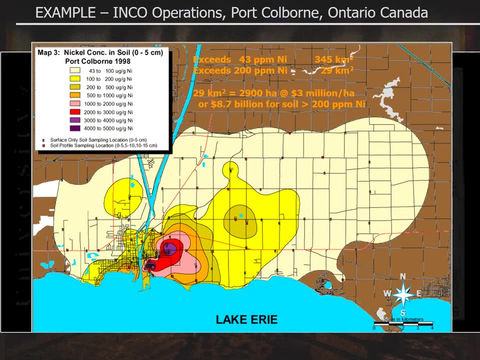 that takes care of whatever contaminants have moved. So an example of this was Inco Operations in Colborne, Ontario, Canada. Here's the site which basically had a nickel contamination related to Inco Operations And they had well over 200 parts per million nickel. 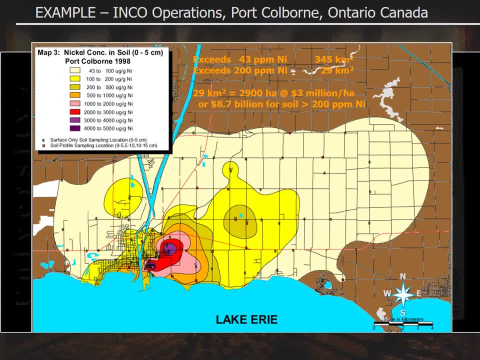 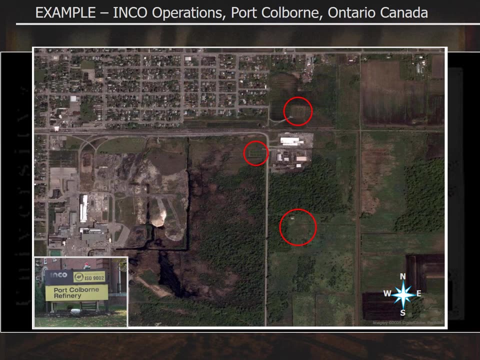 And we're looking at about eight point seven billion dollars for soil decontamination in areas where they had more than 200 parts per million nickel. All right, And so this is on the northern side of Lake Erie, And where these purple or darker spots are is where they had the worst contamination. 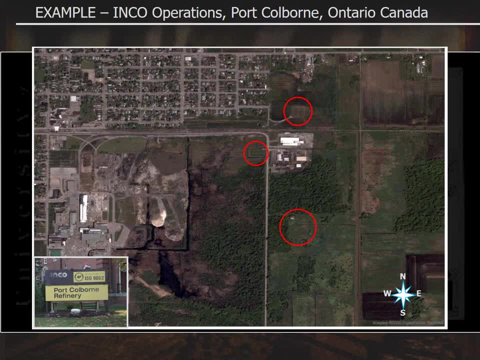 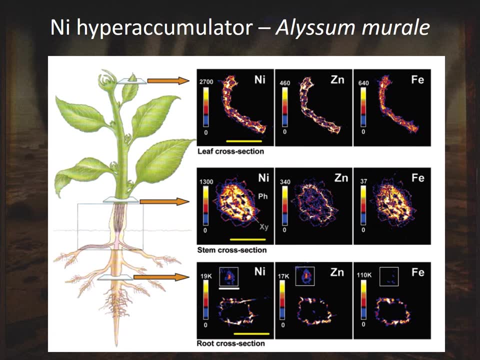 So here you can see the circled areas where we had the highest levels that needed to be addressed. This plant was able to suck the nickel out of the soil and it was a cheaper way to remediate the site. Now remember, these plants were stocked full of nickel.